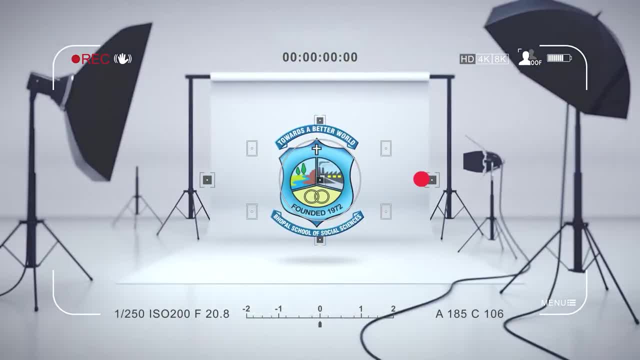 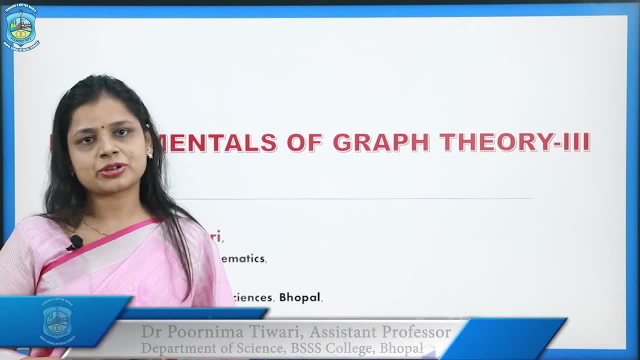 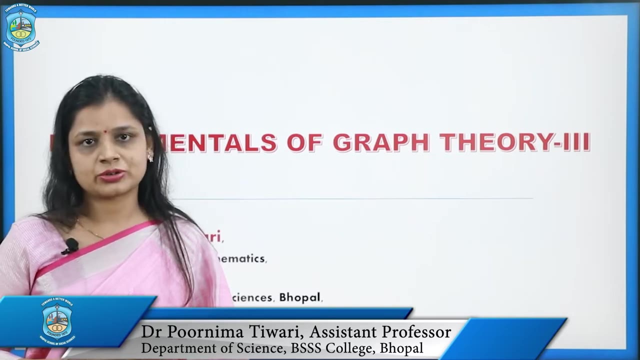 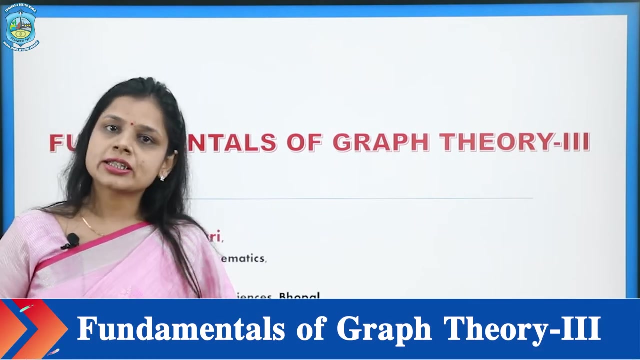 Hello everyone. I am Dr Purnima Tiwari, Assistant Professor of Mathematics Department of Science, the Bhopal School of Social Sciences. In previous video for this topic, Fundamentals of Graph Theory, we discussed several properties and types of graph. In today's video, we will 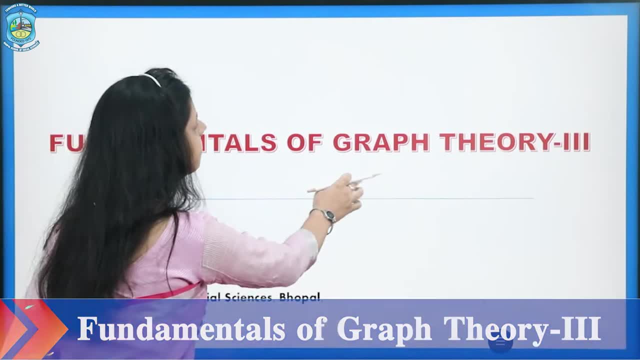 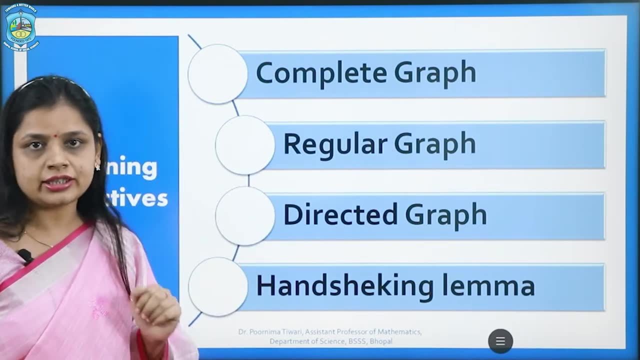 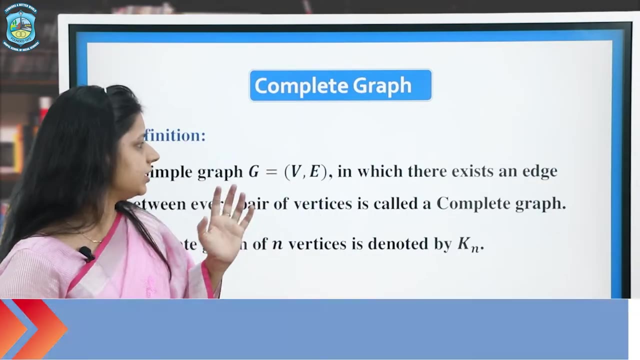 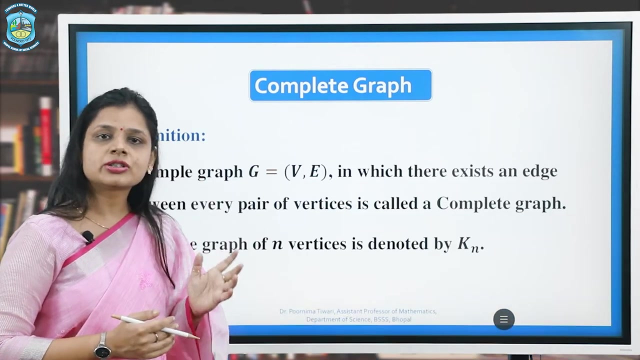 continue with the same topic, and here we will discuss about complete graphs, regular graphs, directed graph and handshaking lemma. Let us start with the definition of complete graph. A simple graph G in which there exists an age between every pair of vertices, is called a complete graph. Here you must note down that this concept is defined. 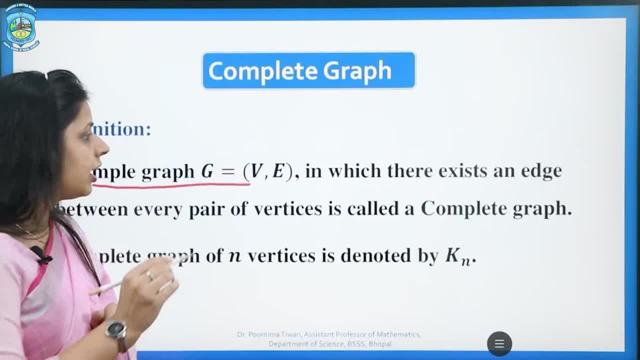 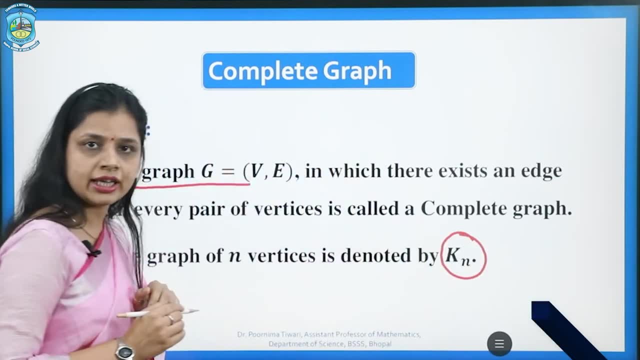 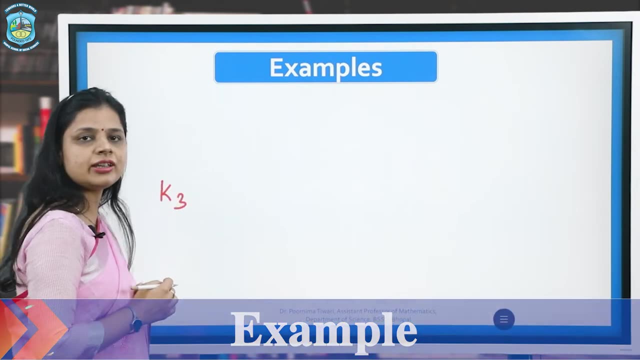 only for a simple graph, And if we have a complete graph of n vertices, we denote it by k n. Let us draw some complete graph. If we have to draw complete graph of three vertices, that is k 3.. So first we will draw three vertex. 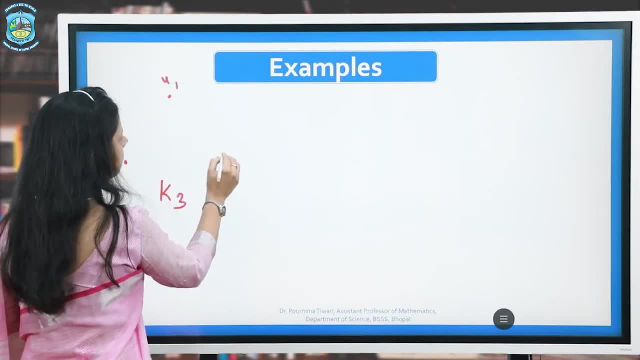 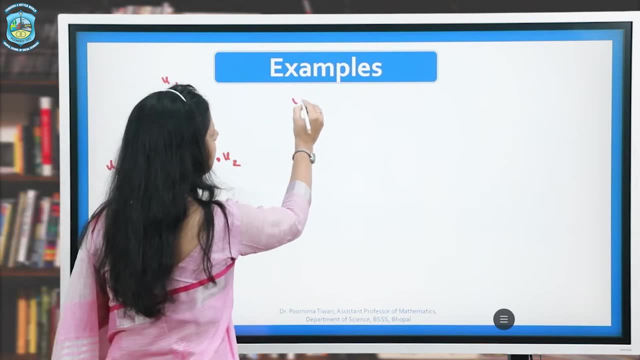 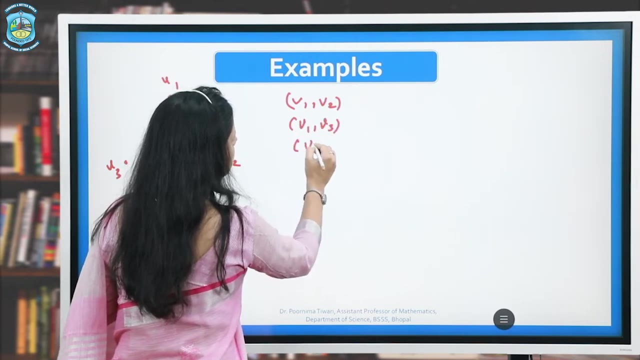 And we may label them as v 1, v 2, v 3.. Now you can see that there are three pair of vertices. One is v 1, v 2.. Second one is v 1, v 3.. And the third one is v 2, v 3.. 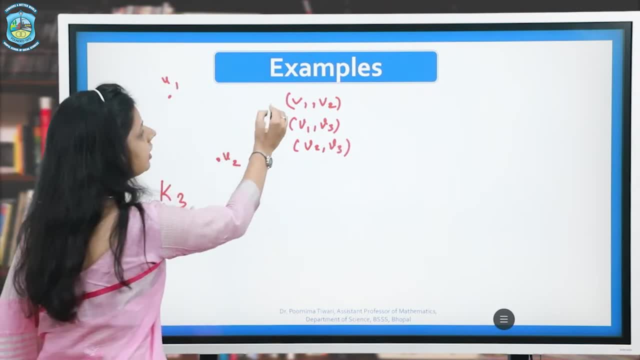 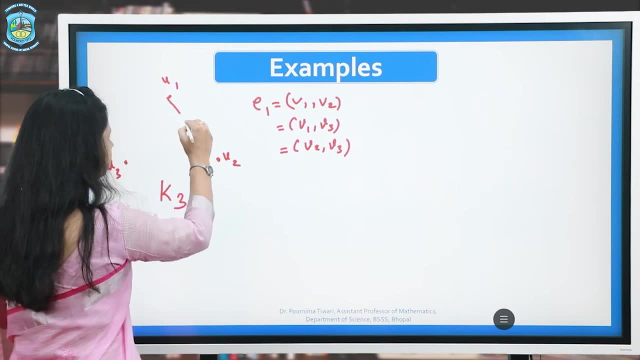 So we have to draw age between each pair of vertices. Suppose we draw e 1 between v 1, v 2. Ah, e 2 between the vertices v 1, v 3. And age e 3 between the vertices v 2, v 3.. 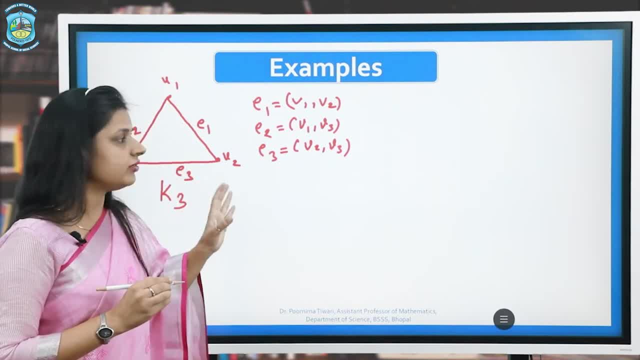 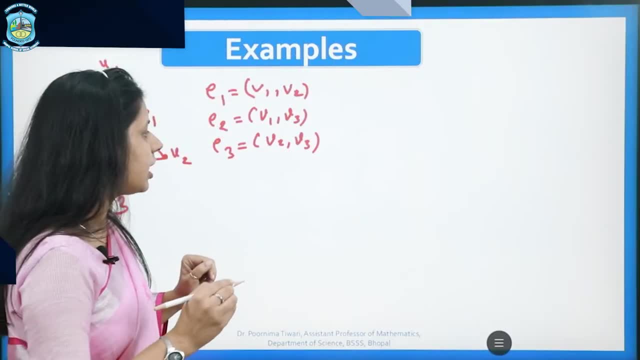 You can see, there is an age between every pair of vertices. So this is complete graph of three vertices. Now, if we have to draw k 4, that is k n, v 2, v 3.. Now we have to draw k 3.. And we have to draw k 4,, that is k 3.. So this is a complete graph of three vertices. Now, if we have to draw k 4, that is k n, v 2, v 3.. And we may label them as k 3.. And here you must note them as k 2, v 3, v 2, v 3.. And again, when we have to draw k 4, there is a complete graph of a combo of ethics: времени, travel, time, variations, time counting. 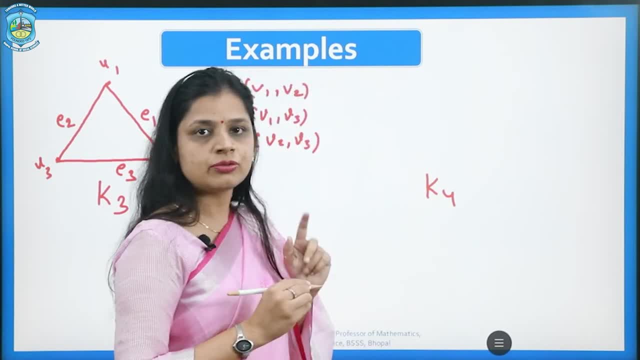 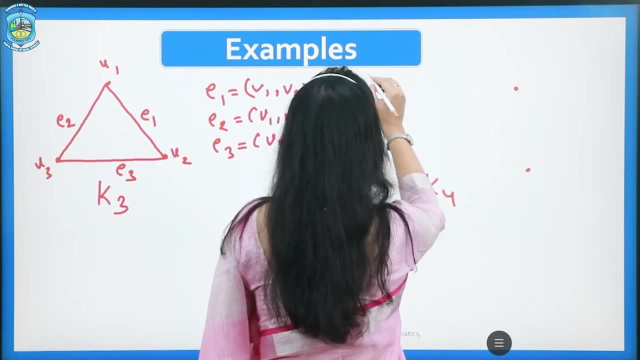 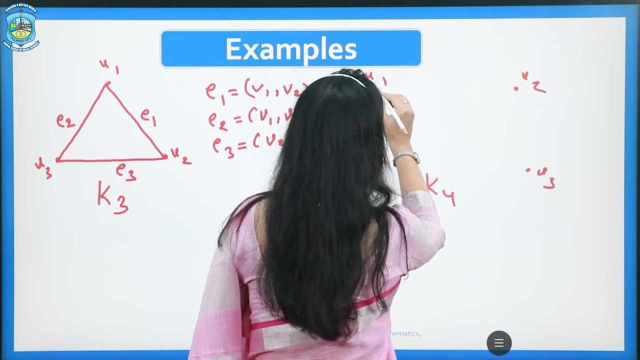 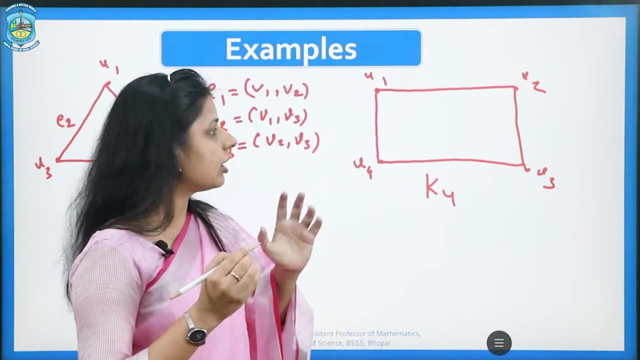 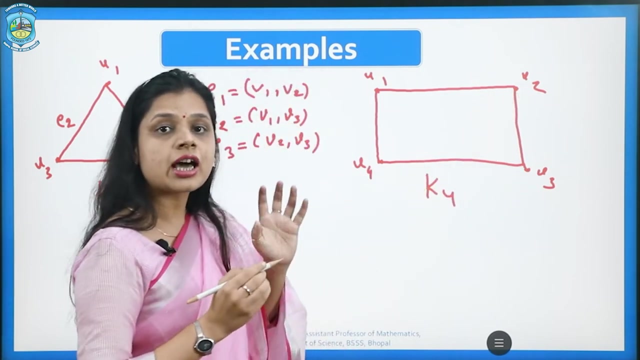 draw K4. that is complete graph of four vertices. So first we will draw four vertex, then we can draw either a rectangle or I square joining these four vertices. Now you can see that there is two pairs, V1, V3 and V2, V4, which are not joined by an edge. So for the complete, 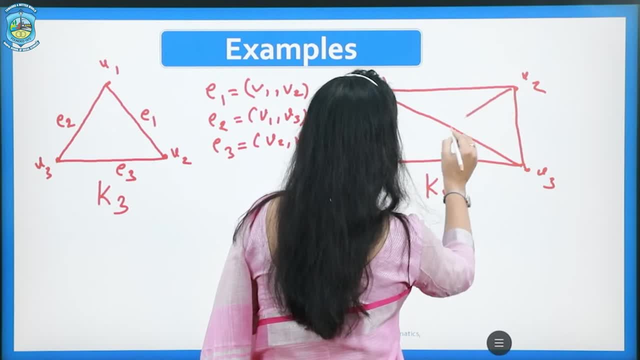 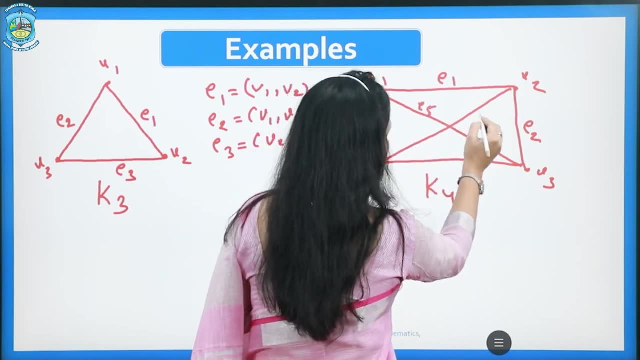 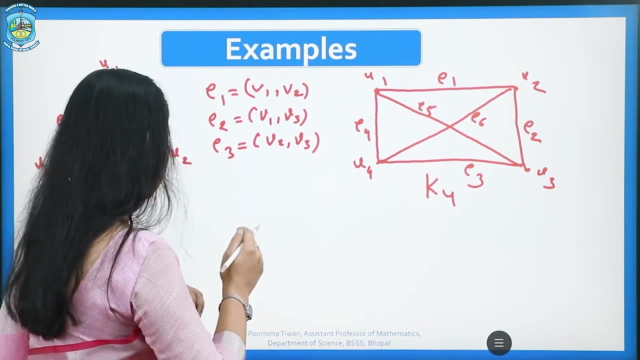 graph. we have to join these two pairs. We may label the edges E1, E2, E3, E4, E5 and E6.. So this is complete graph of four vertices. If we have to draw complete graph of five vertices, 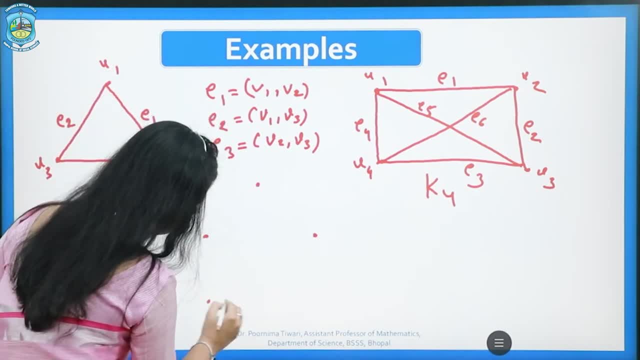 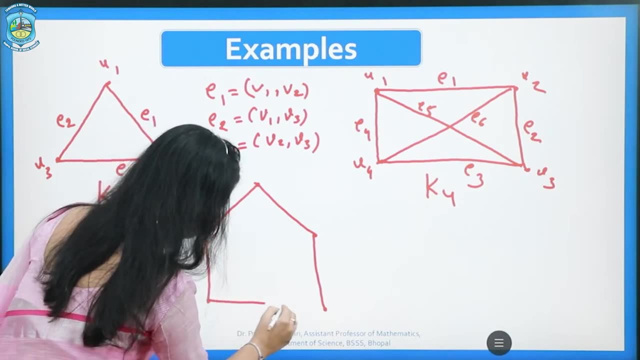 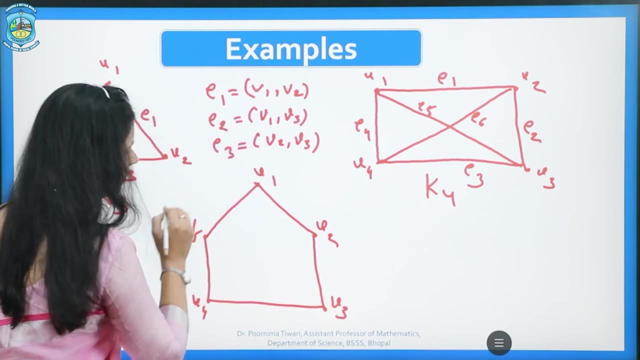 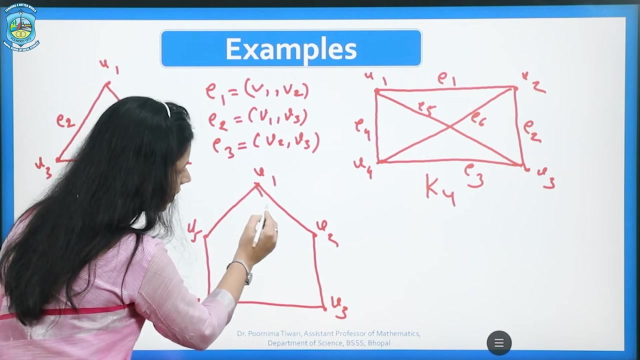 First we need to draw a pentagon. We may label vertices V1, V2, V3, V4, V5.. Now we have to draw an edge between every pair of vertices. So we have to connect V1 and V3, V1 and V4,. 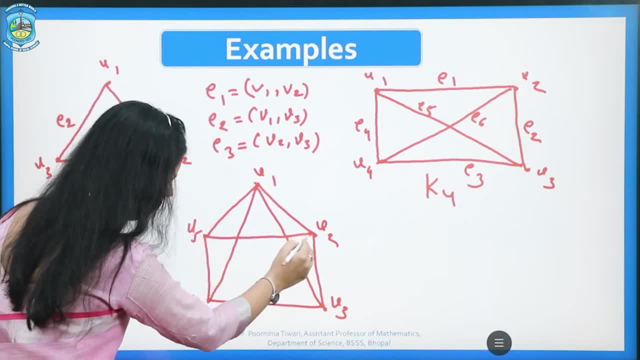 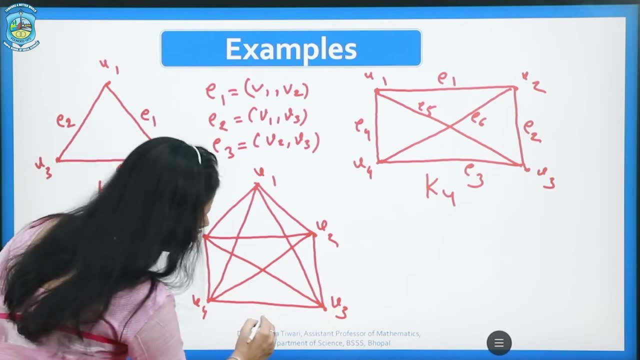 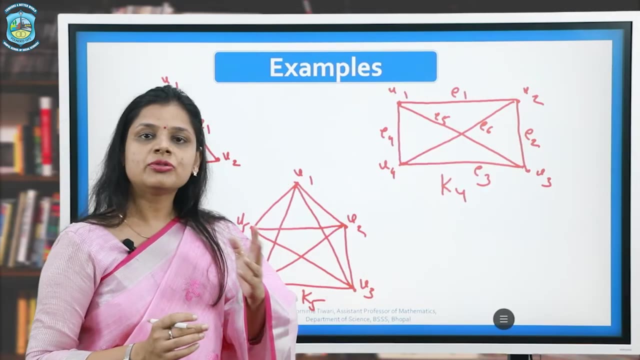 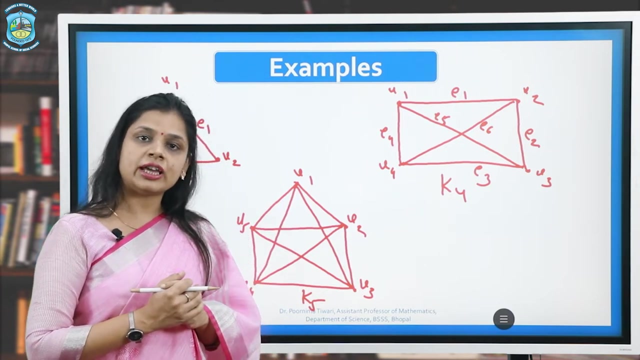 V2 and V5, V2 and V4 or V5 and V3.. So this graph is a complete graph of five vertices. We denote it by K5.. Now we have two important observation regarding complete graph. First, that the complete graph of n vertices has n n minus 1 by 2 edges. 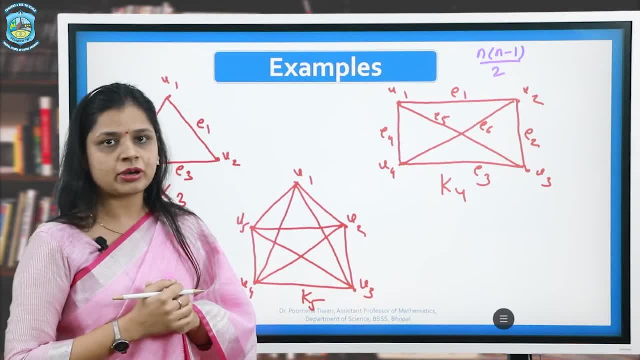 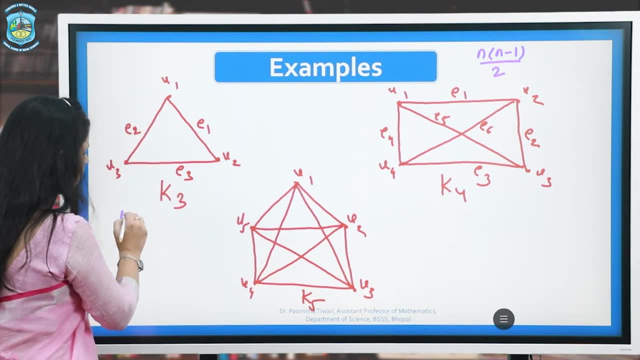 That is k? n has n? n minus 1 by 2 edges. We may verify with the example here for the Kme, pour yang 3 numbers of vertices are 3.. If we calculate this Dom and n? n minus 1 by 2 will get 3 into 2 by 2.. So we will get 3 and Kmeximize and we can verify. There are. 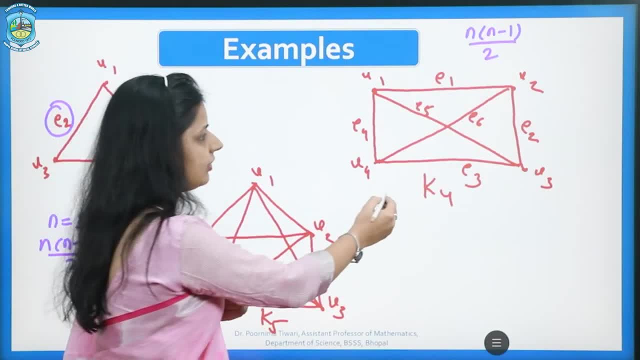 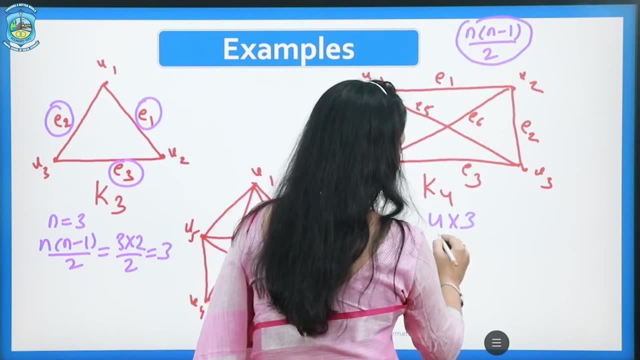 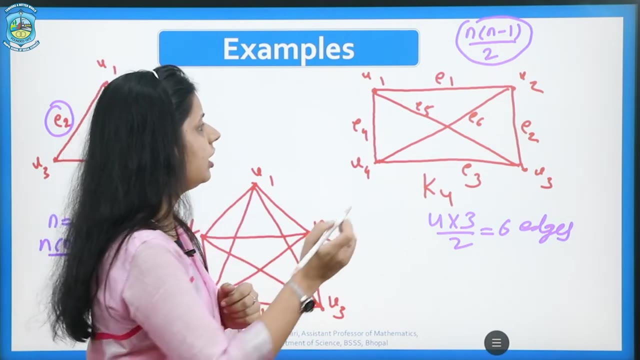 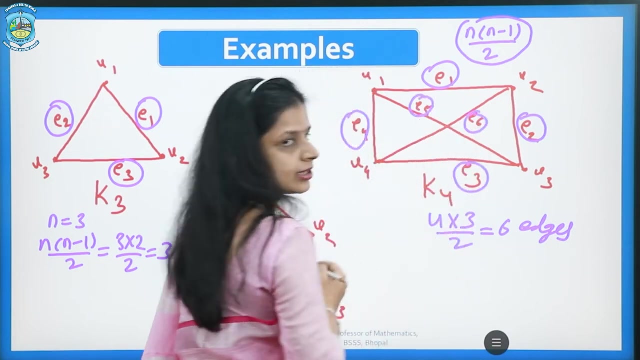 3 edges in K3.. for K4. If we apply this rule for K4, we will get 4 into 3 by 2, that is 6 edges. So K4 must have 6 edges as per this rule and we can see there are 6 edges: E1, E2, E3, E4, E5, E6. 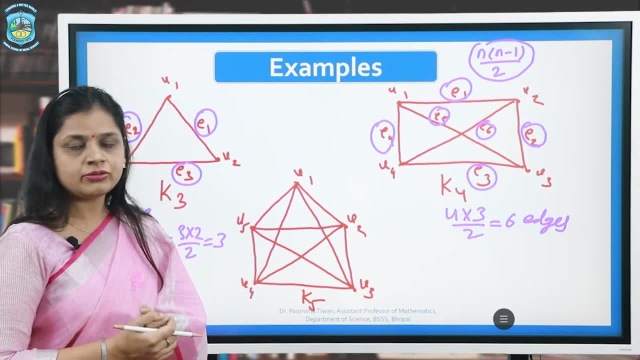 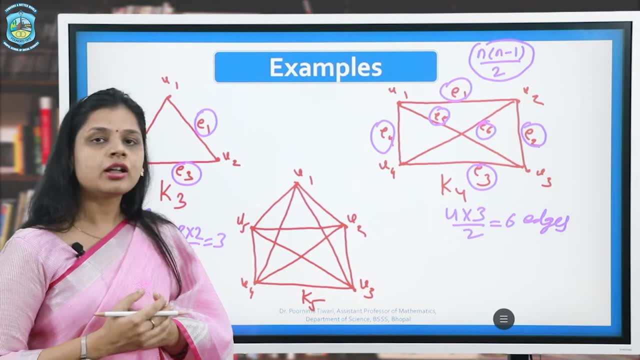 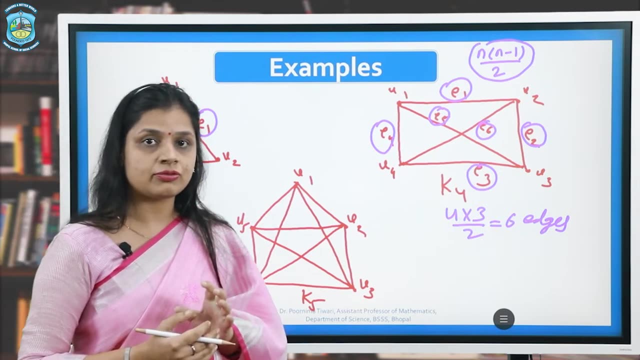 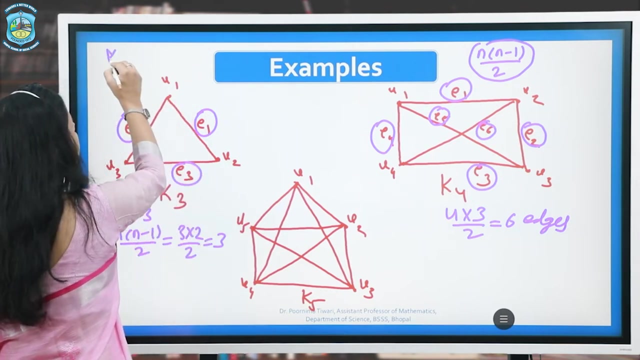 Likewise we can verify this result for K5.. For better understanding, you may draw K6 and may verify this result. Second observation is that degree of every vertex in a complete graph of n vertices is n minus 1.. That is, if we have this Kn, then the degree of every vertex will be: 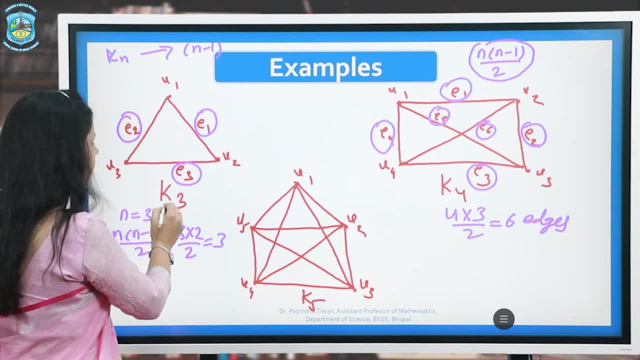 n minus 1.. We can verify. See this in this graph. we have K3 and if we calculate degree of V1, it will be n minus 1.. So we can verify this. So we can verify this. So we can verify this. 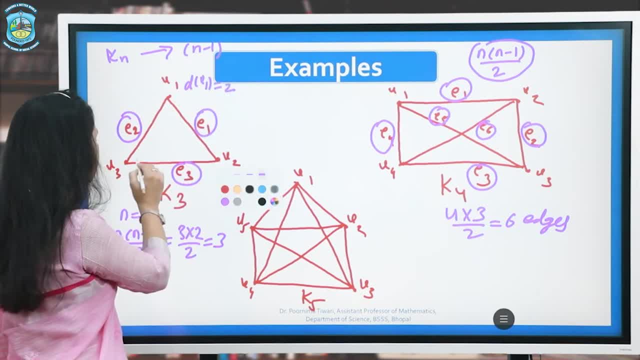 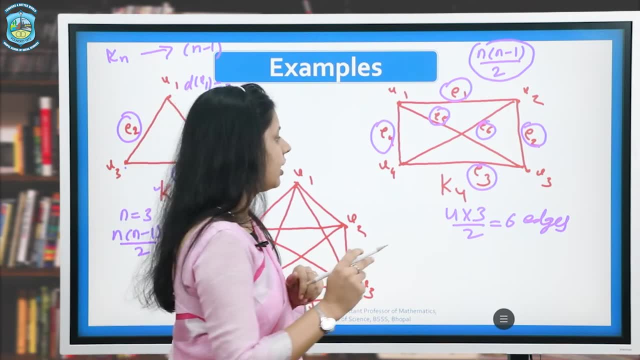 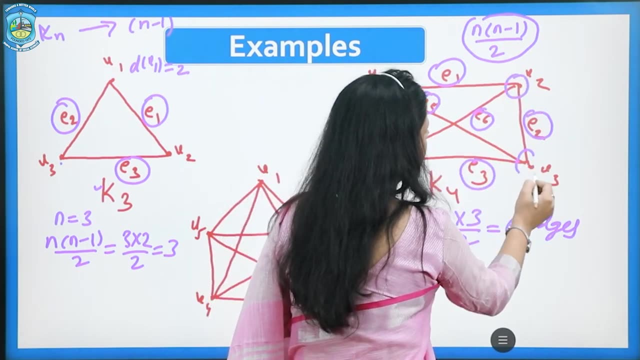 It is 2.. Likewise, degree of V2 is 2 and degree of V3 is 2.. So in K3 degree of every vertex is 2.. If we see this example K4, we can see degree of every vertex is 3.. V1, V2, V3, V4.. All the 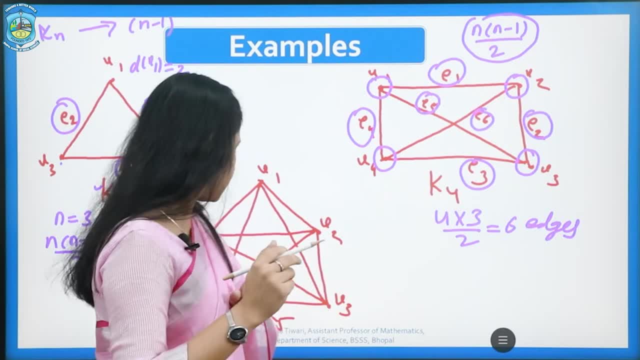 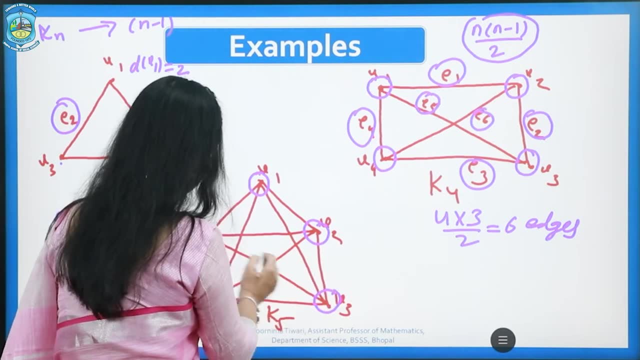 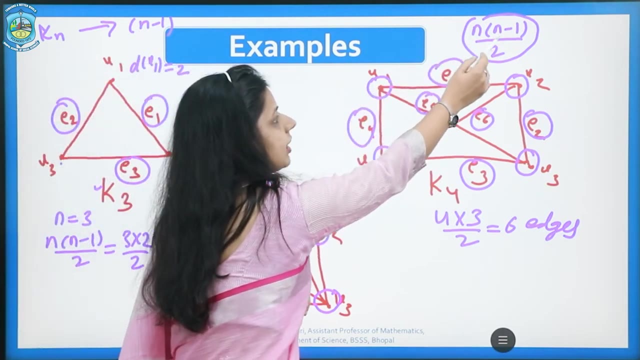 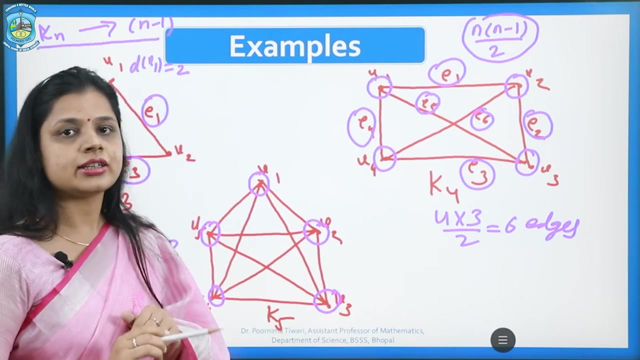 vertices are of degree 3.. Similarly, if we talk about this K5, you can see degree of every vertex is 4.. So these are two important observation: that Kn has n n minus 1 by 2 edges and the second thing, degree of every vertex in Kn is n minus 1.. Next definition is for regular graph. 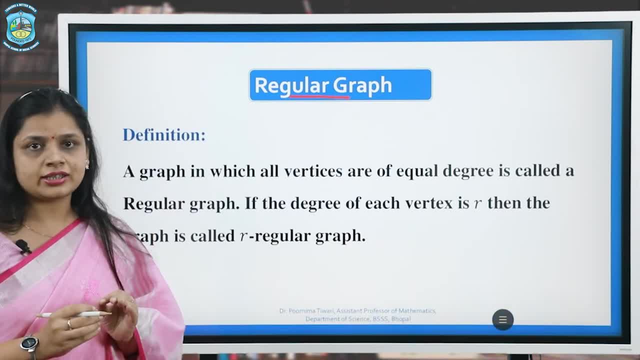 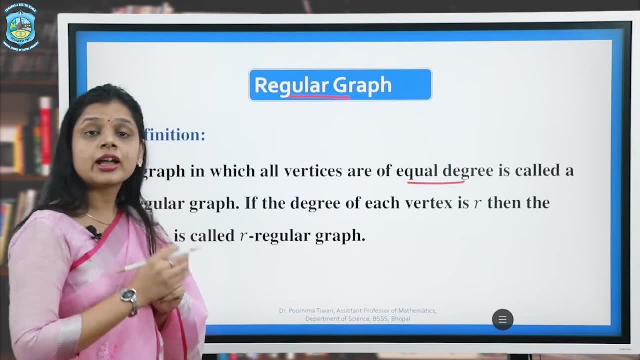 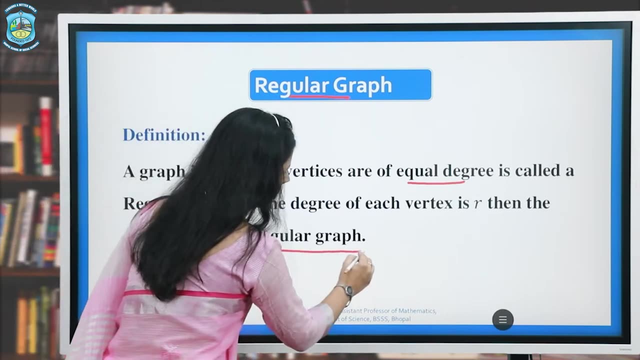 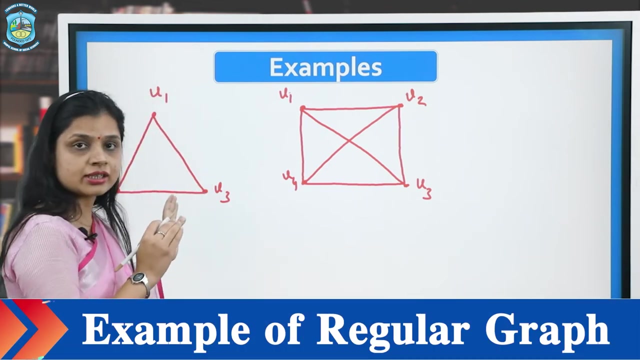 A graph in which all vertices are of equal degree is called a regular graph, And if degree of each vertex is R, then the graph is called R- regular graph. Now in the examples of regular graph we can see that the previous graph that we draw for complete graph are also regular. 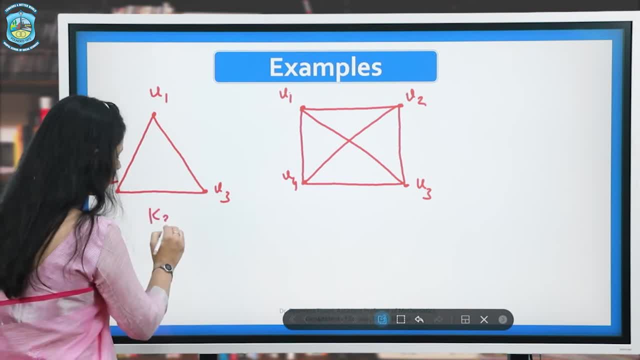 graph. So if we talk about this K3 complete graph of three vertices, you may notice that the degree of each vertex is 2.. Degree of V1 is 0.. Degree of V2 is 0.. Degree of V3 is 0.. Degree of V3 is 0.. 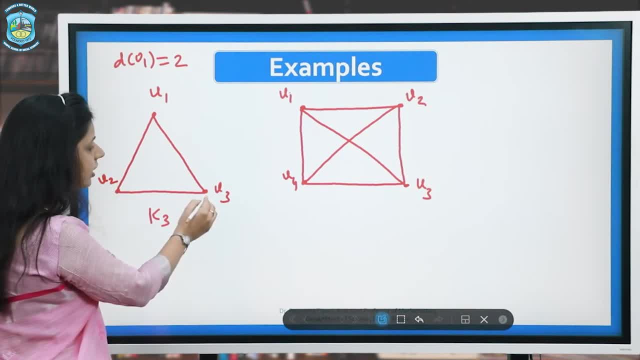 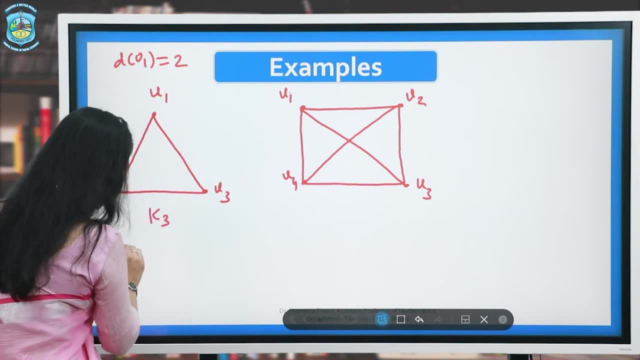 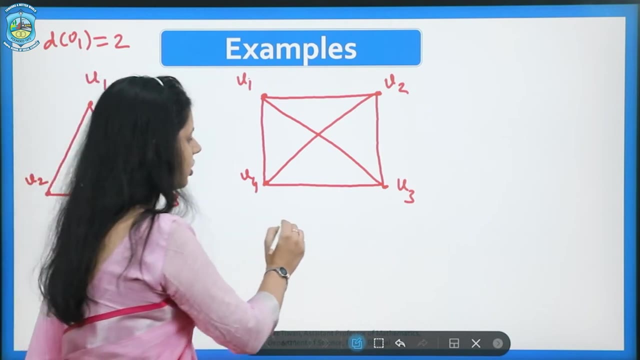 V1 is 2. likewise degree of V2 is 2 and degree of V3 is 2.. It means in K3 every vertex is of degree 2. that's why this K3 is 2 regular graph And if we talk about K4 we may notice that degree of. 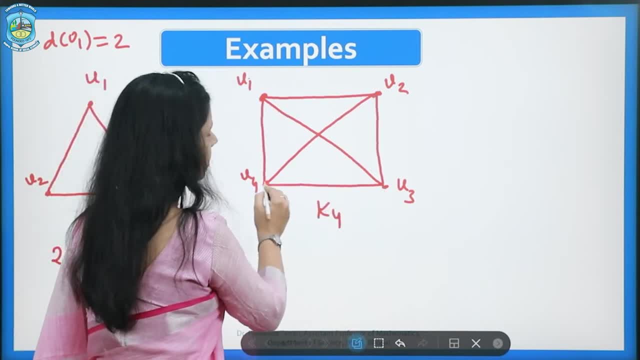 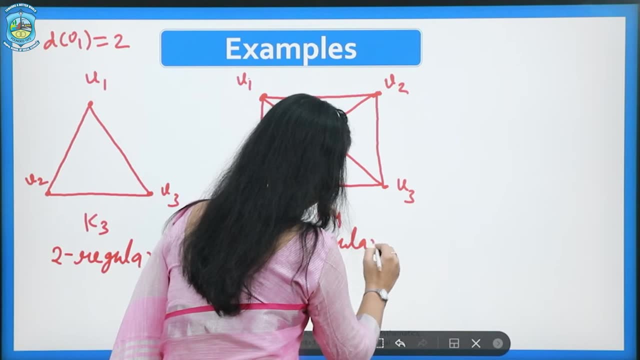 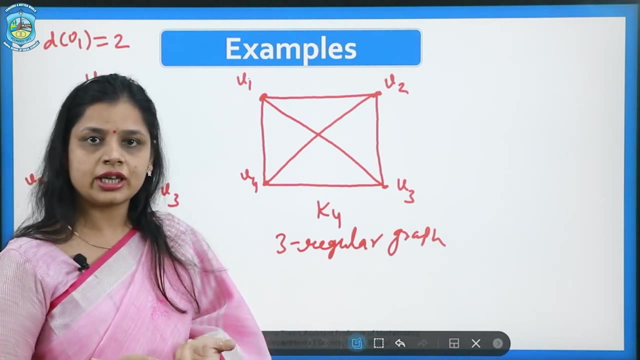 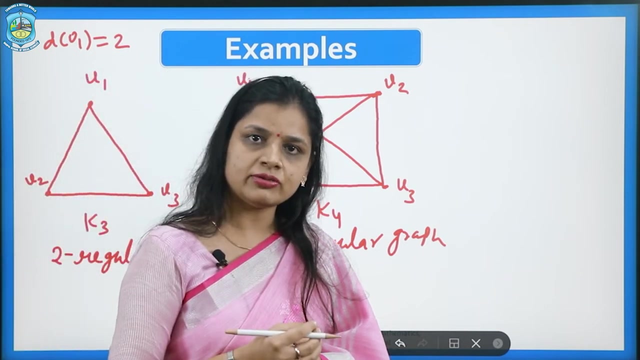 each vertex V1,, V2,, V3, V4 is 3.. So this K4 is 3 regular graph. Likewise, if we talk about K5, it is 4 regular graph. So we can say that every complete graph of n vertices is n minus 1 regular graph. 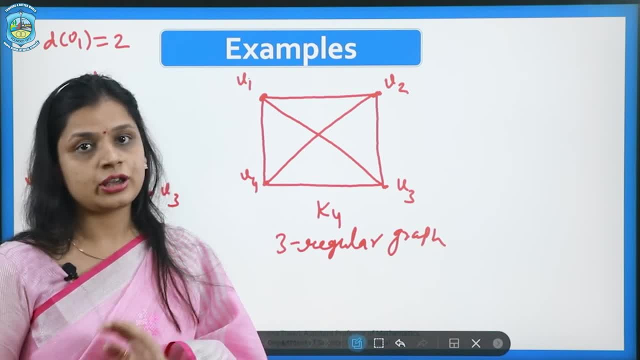 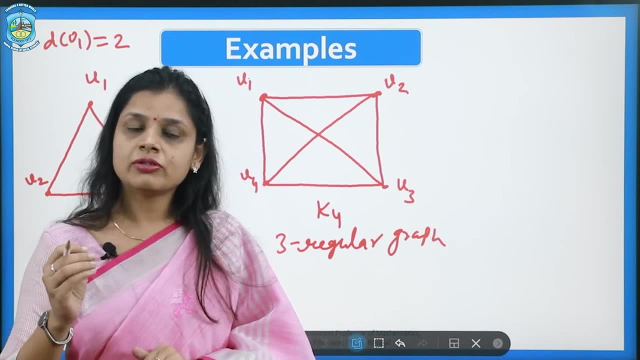 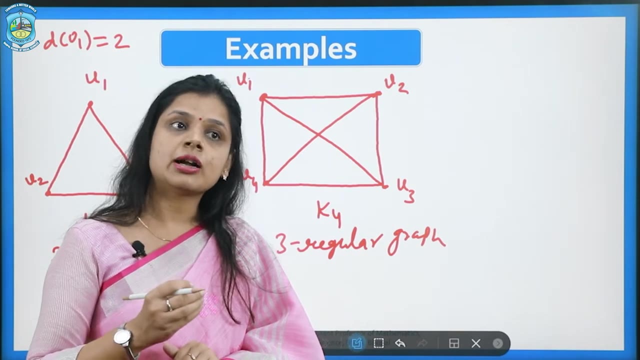 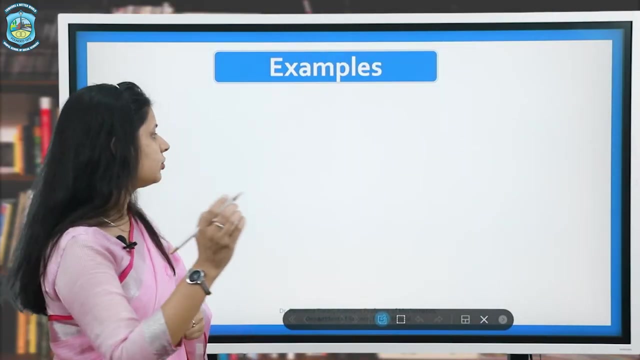 It means every complete graph is a regular graph, but converse of this statement is not true. We can always draw a graph which is regular but not complete. Its example is one of the famous graph known as Kuratowski's 2 graph. Now to draw this Kuratowski's graph. it's a graph with 6 vertices. and 9 vertices, So we can say that every complete graph is a regular graph. And if we talk about this Kuratowski's graph, its skew is similar to that of 3 ninguém, made of 6 vertices and 9 edges. 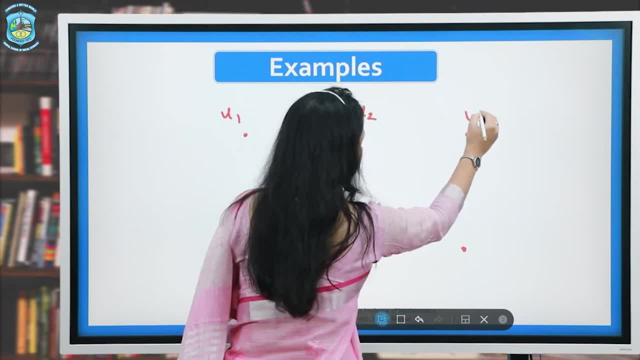 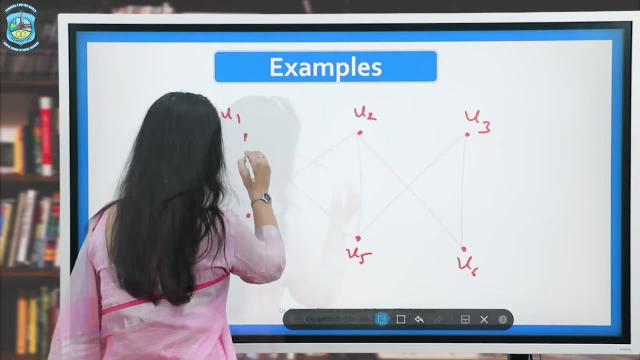 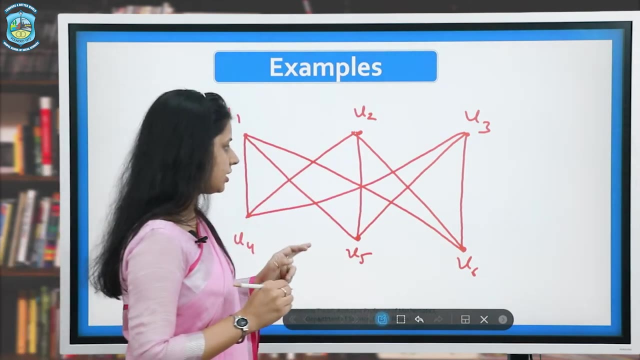 So we may label those vertices as V1, V2, V3,, V4,, V5, V6.. So this is Kuratowski's second graph. It is called as K33.. You can notice that degree of two vertices is a regular graph and the angle of two vertices is 1 and the angle of two vertices is 2.. So we can say that every complete graph is K3.. Likewise, if we talk about K3, every complete graph is asset world. They have all three registers. We can also draw a graph which is V1,, V2,, V3,, V4,, V1, V6.. 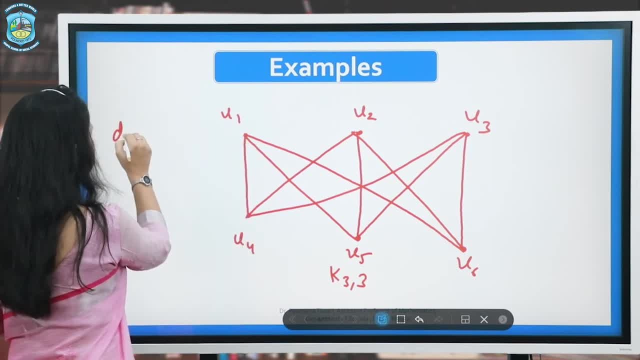 So this is Kuratowski's second graph. It is called as K33.. So these two are all regular laws here: Musikl, Evlle and Kehler, Fried & Groth. Degree of each vertex is 3 here. If we talk about degree of VI, then it is 3, for I varies from 1, 2 up to 6.. 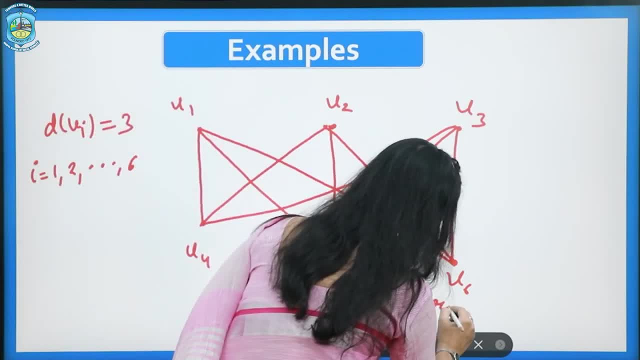 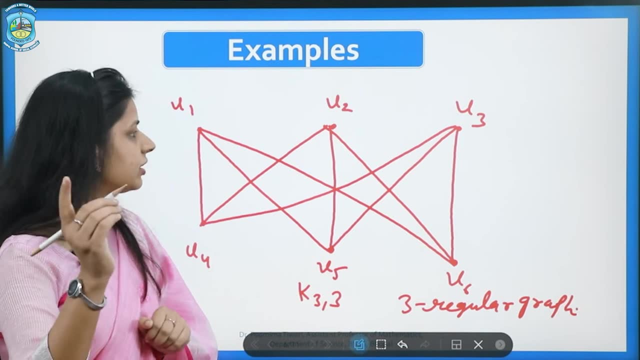 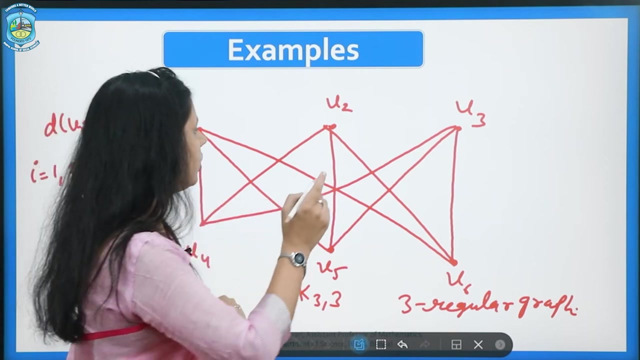 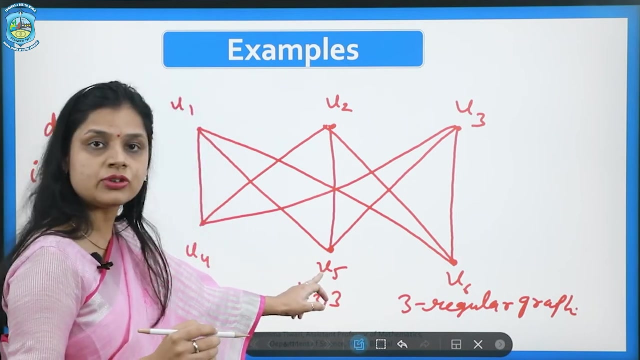 So this graph is a 3 regular graph, But we can see there is no edge joining the vertex V1 and V2.. There is no edge joining the vertices V2 or V3.. Likewise, no edge in between the vertices V4 and V5 or V5 and V6.. 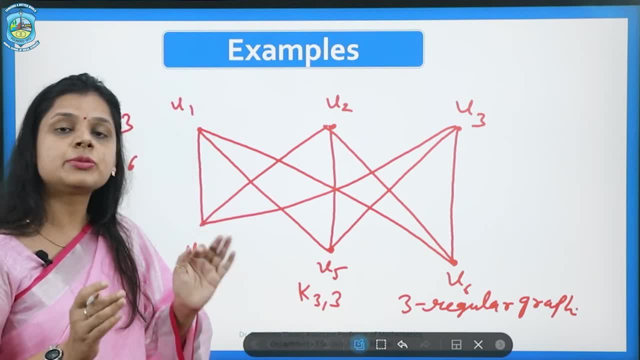 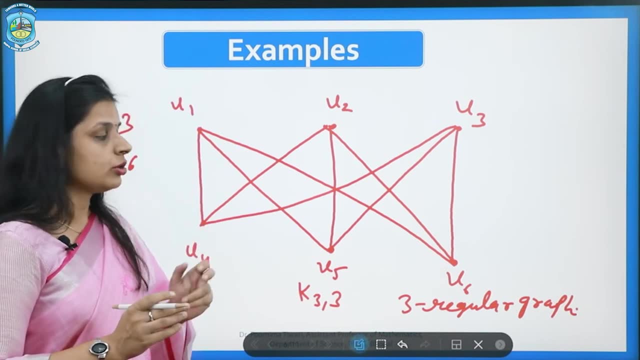 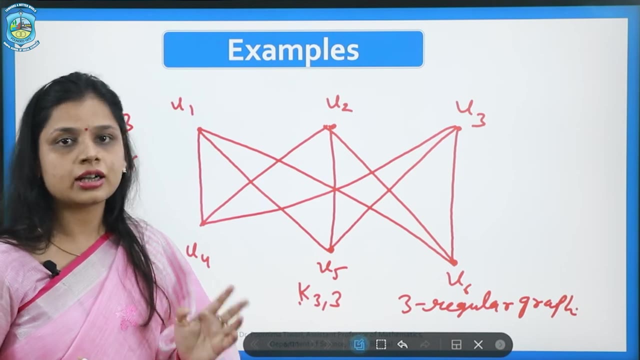 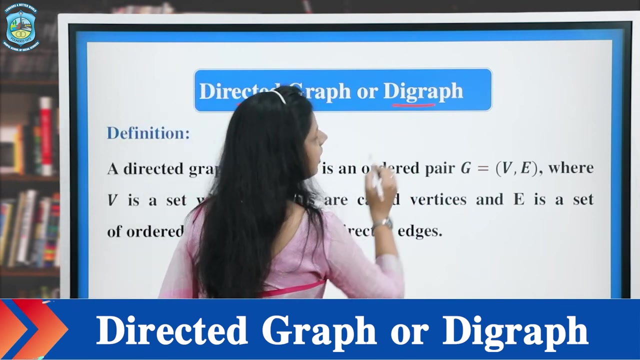 It means there does not exist an edge between every pair of vertices, So this graph is not a complete graph. So if we talk about this graph K33, it is a 3 regular graph, But it is not a complete graph. Next definition is for directed graph, which is also known as digraph. 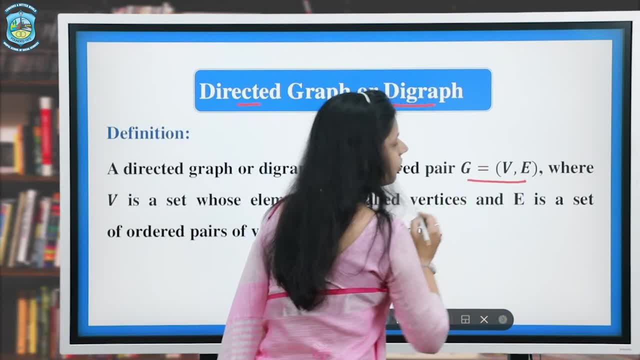 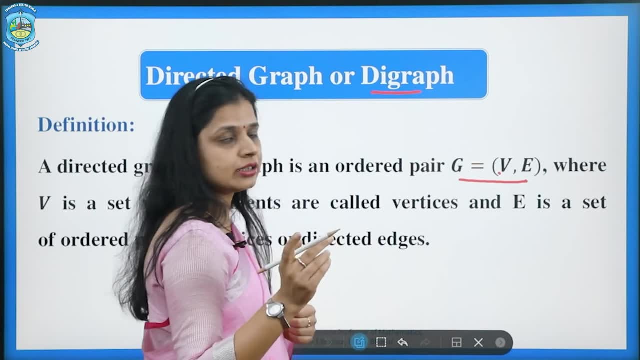 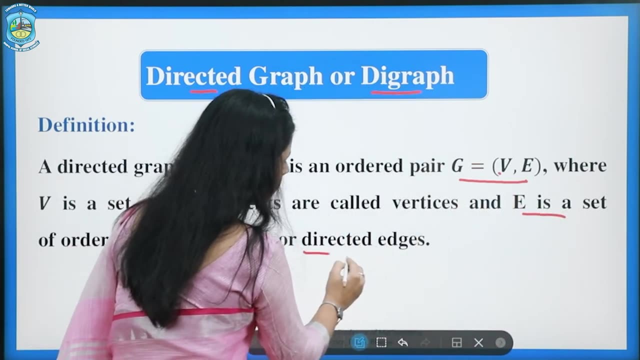 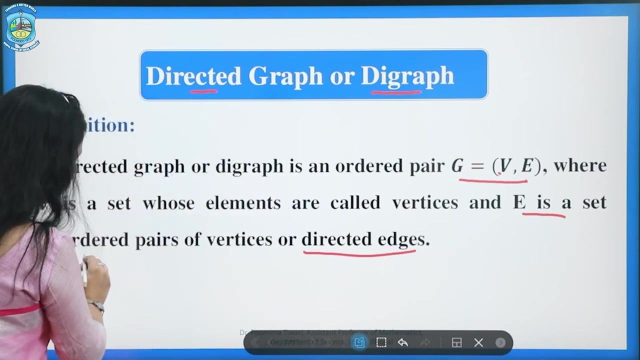 A graph G is equal to VE is called a directed graph or digraph. If this V is same as in the case of undirected graph, it is set of vertices, But this set E is the set of directed edges. Or we can say that this set E is the set of ordered pair of vertices. 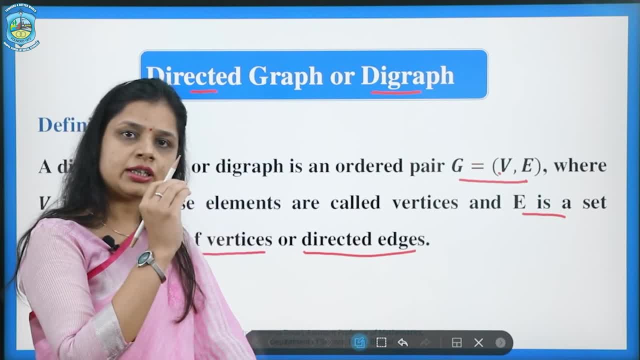 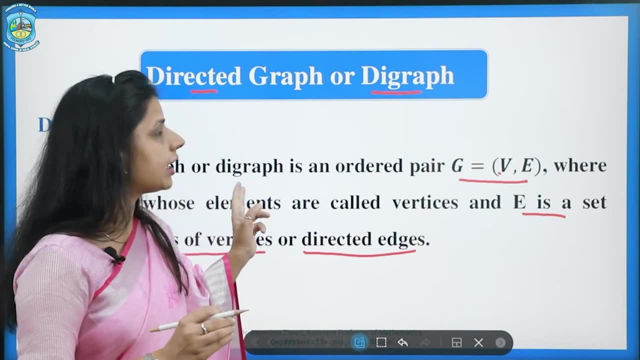 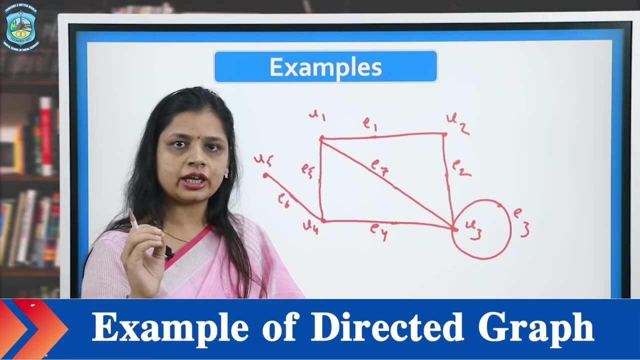 It simply means that if in the undirected graph we assign a direction to each edge, then the graph become directed graph or digraph. For the example of directed graph: first we can draw an undirected graph as this graph. This is the undirected graph. 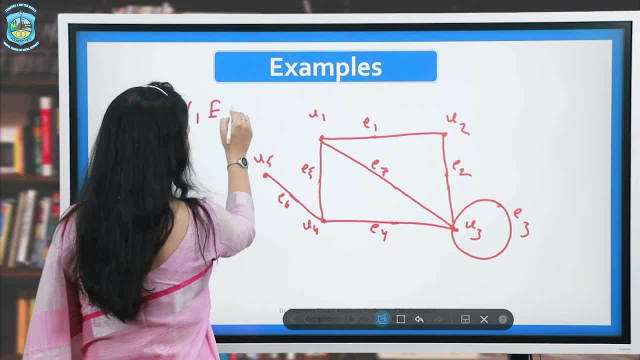 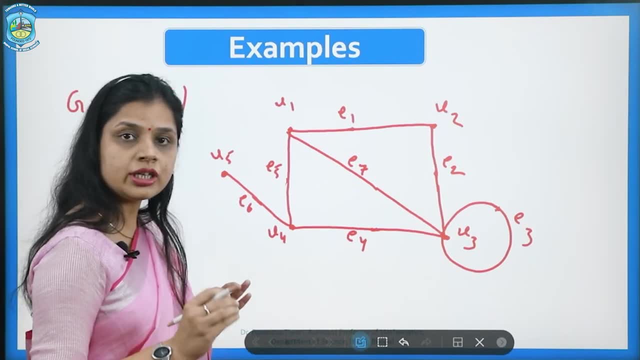 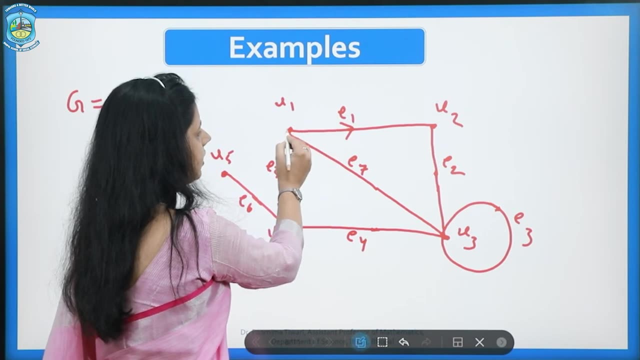 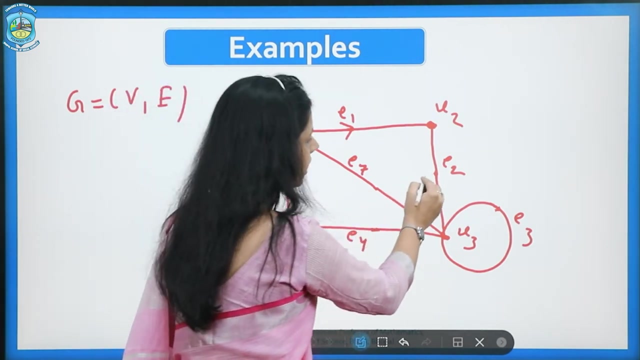 graph G is equal to VE, with 5 vertices and 7 edges. Now if we assign a direction to each of its edge, like this direction to edge E1, that is, this edge E1 is started with the vertex V1 and terminated at the vertex V2.. We can assign any direction, either in clockwise or 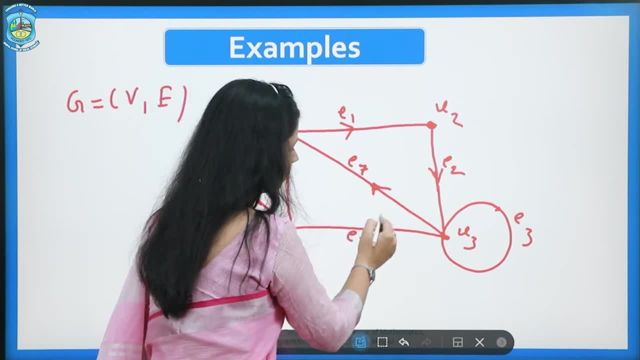 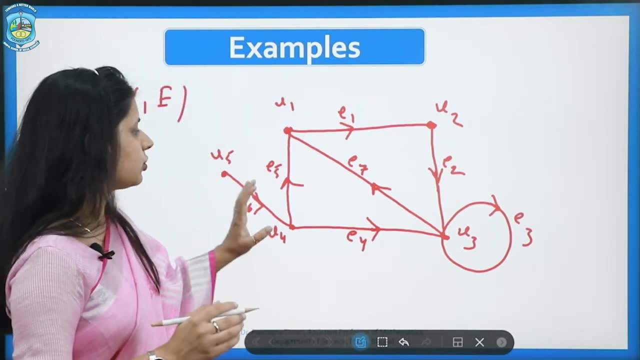 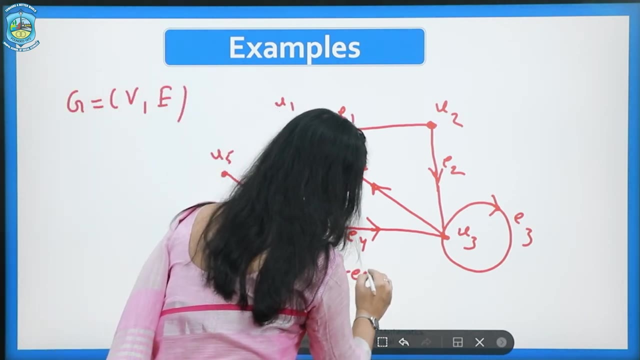 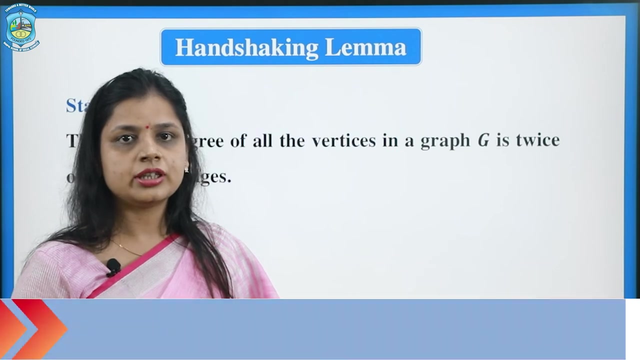 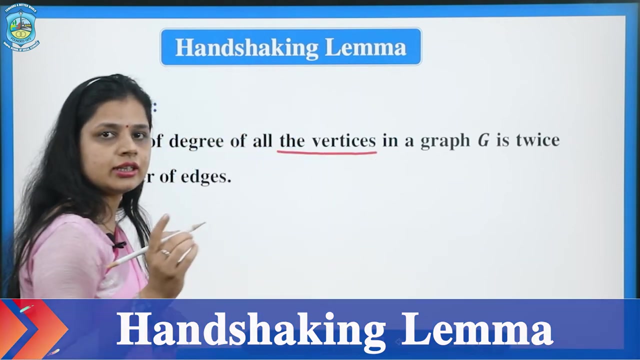 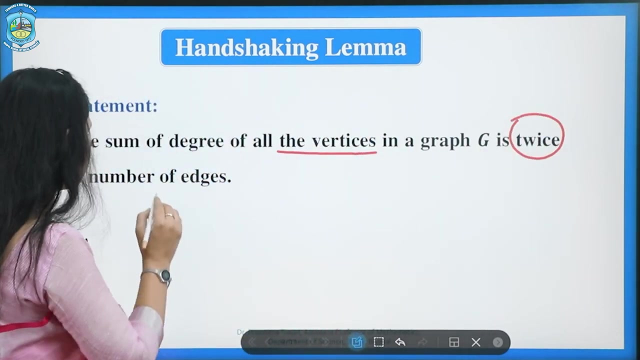 in anti-clockwise to each edge. So I assign a direction to each edge. So now this graph is a directed graph. Next concept is handshaking lemma. It is stated as the sum of degree of all All the vertices in a graph is twice of number of edges. So suppose, if we have this graph, 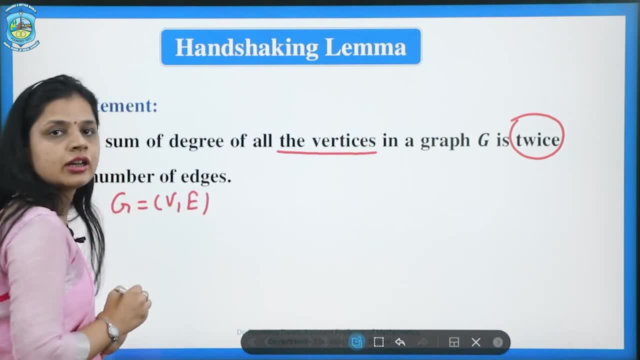 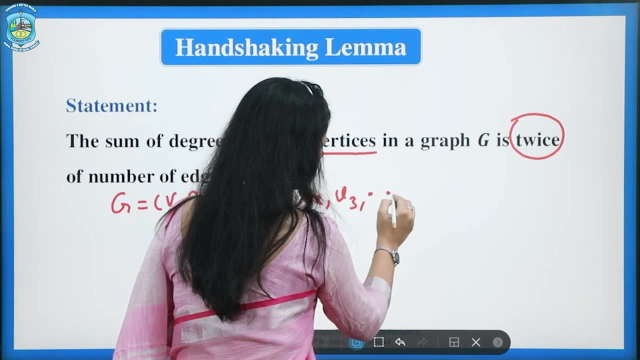 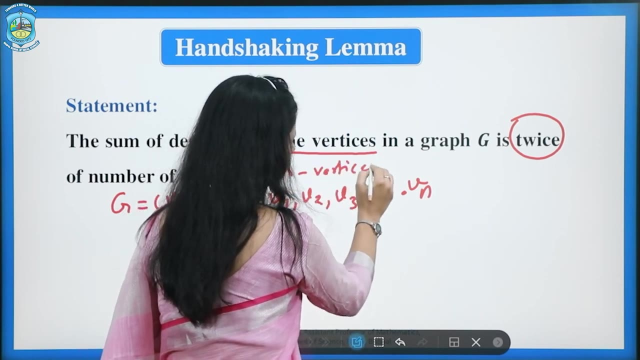 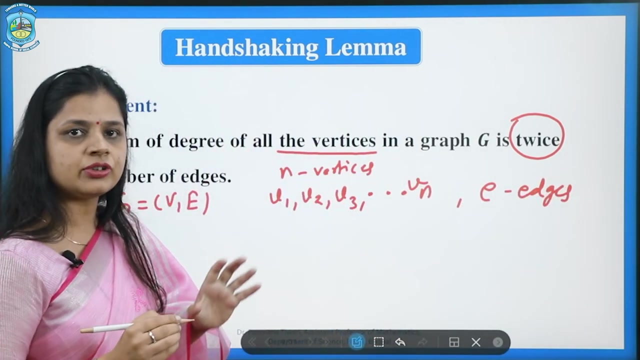 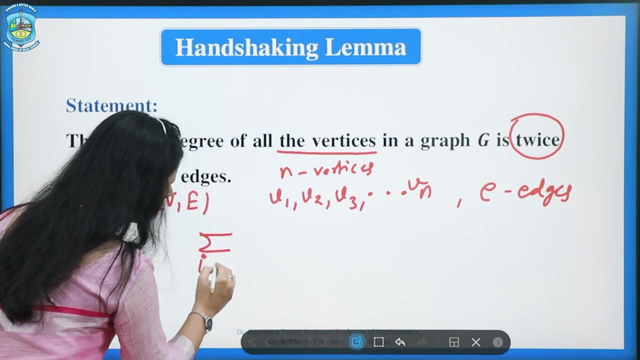 G is equal to VE and this graph has n vertices: V1,, V2, V3, up to VN. These are n vertices and E8. So we consider a graph with n number of vertices and E8. Then this lemma said: summation I varies. 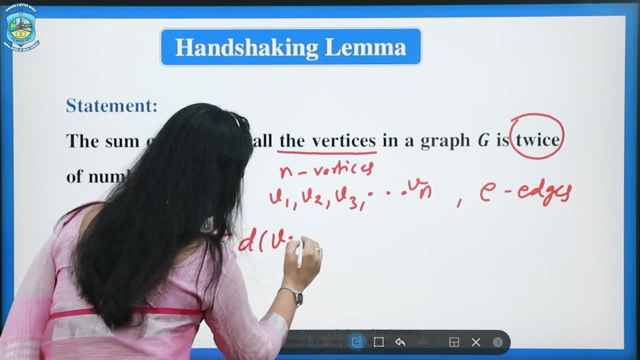 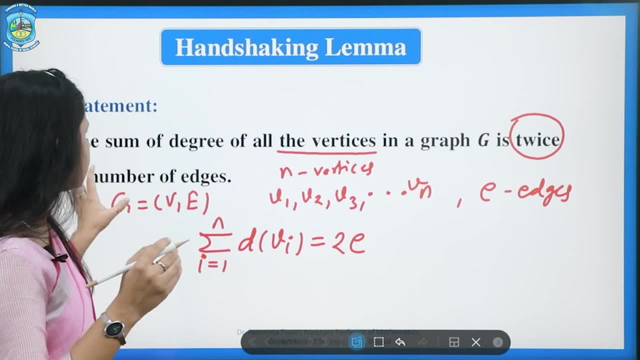 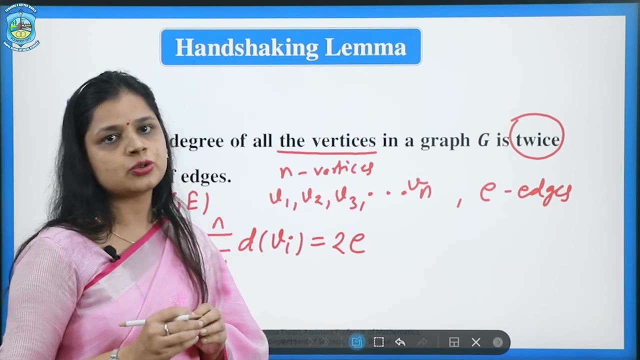 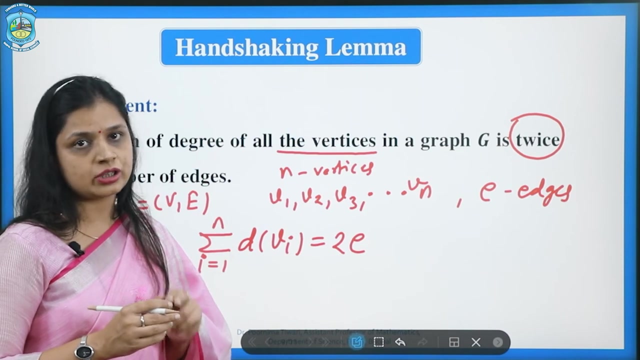 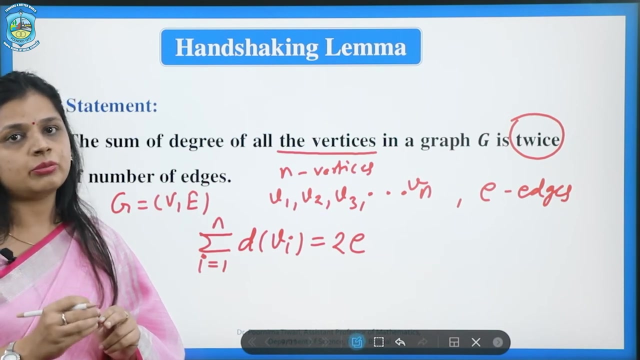 from 1 to N D of VI is equal to twice. We can prove this lemma by simple using one argument: that each edge incident on exactly two vertices, That is, each edge contributes to the sum of degree of vertices. So whenever we get sum of degree of vertices, it will be twice of number of edges. We may verify handshaking. 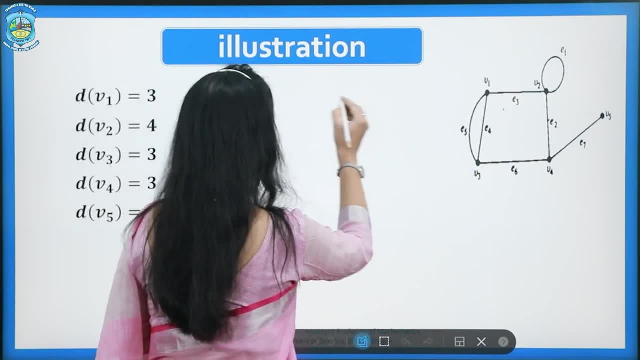 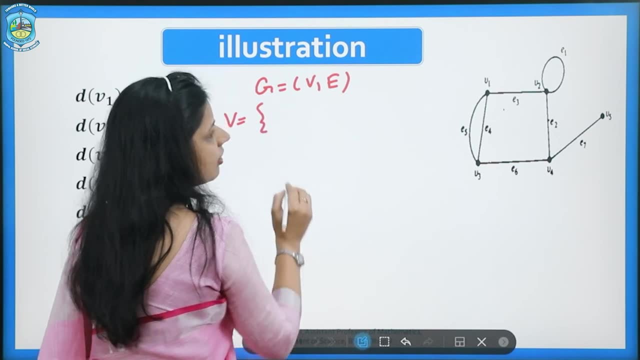 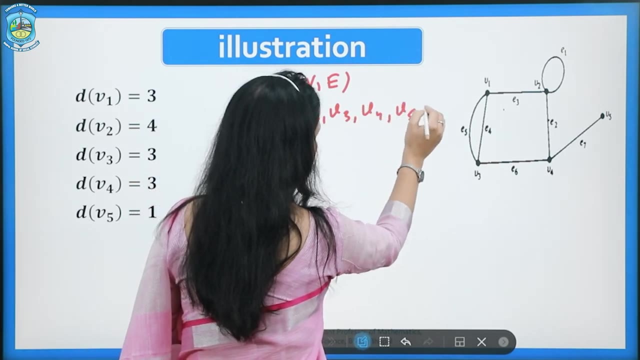 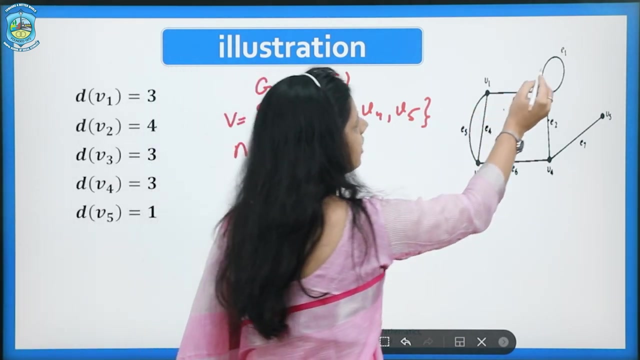 lemma for any graph. Suppose I consider this graph G is equal to VE, where it has five vertices: V1, V2, V3, V4, V5. that is, n is equal to 5. And the set of edges has elements E1,, E2,. 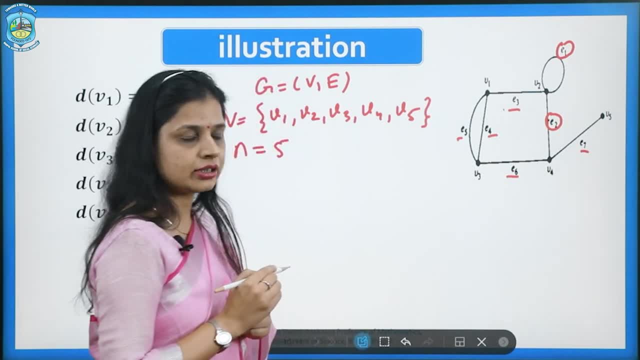 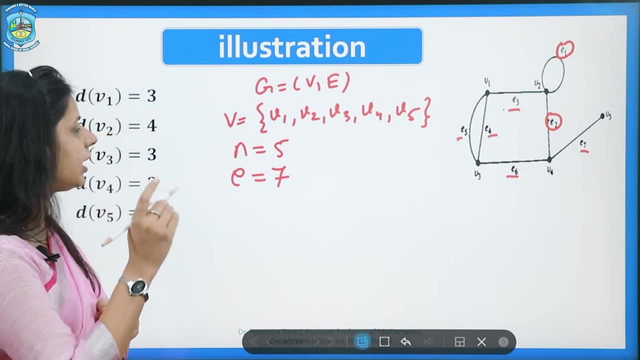 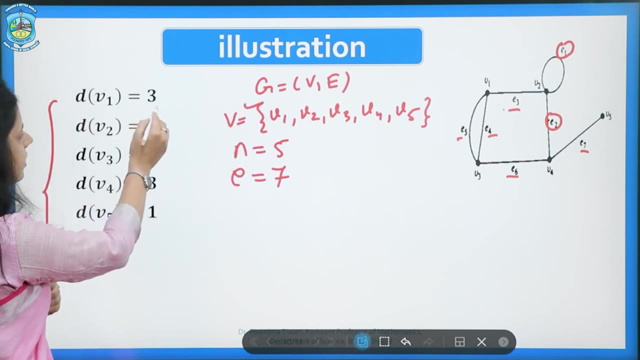 E3, E4, E5, E6 and E7, that is, number of edges, are 7.. Now, first we have to calculate degree of each vertex, and we find that degree of V1 is 3,, V2 is 4, V3 is 3,, likewise V4 is.